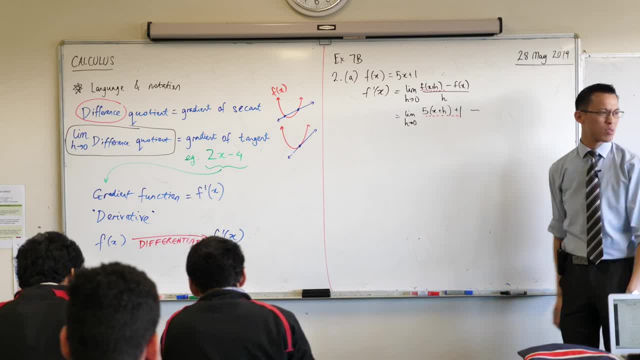 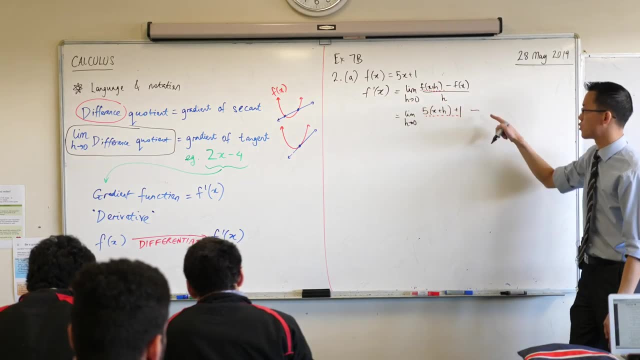 So that's good. Take away What's my f of x. Have a look, just by definition It's that guy right Now. just be careful, because I'm subtracting a whole function. I'm going to chuck some brackets in here because there's going to be a minus sign. that sort of distributes. 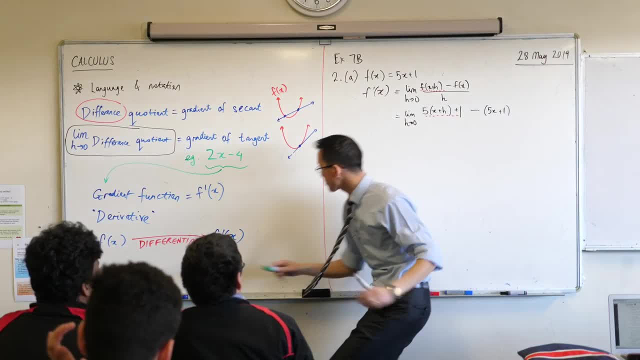 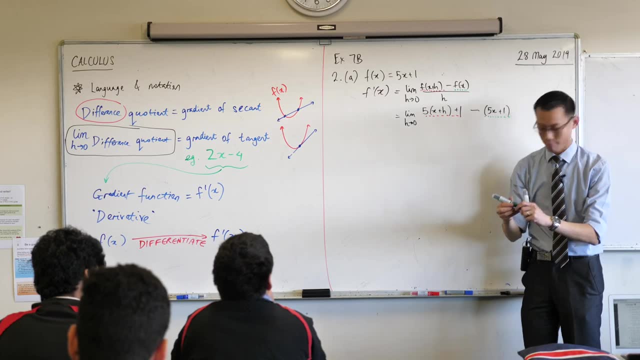 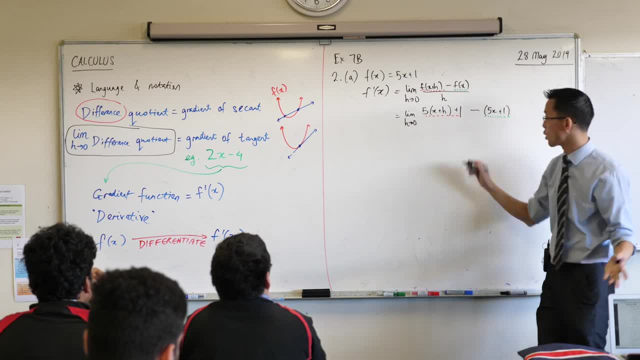 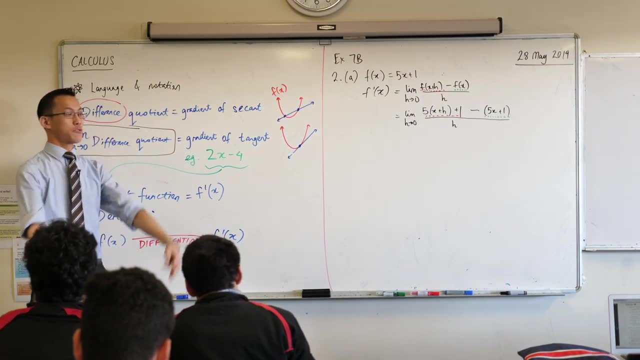 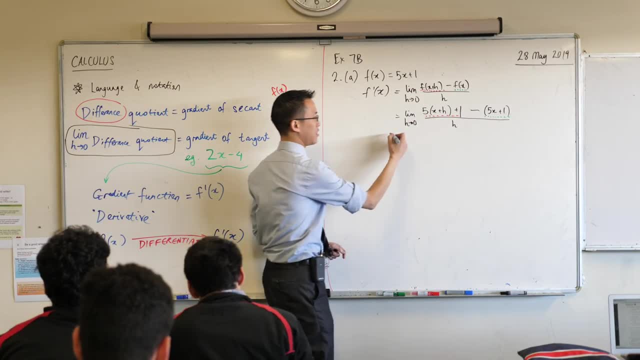 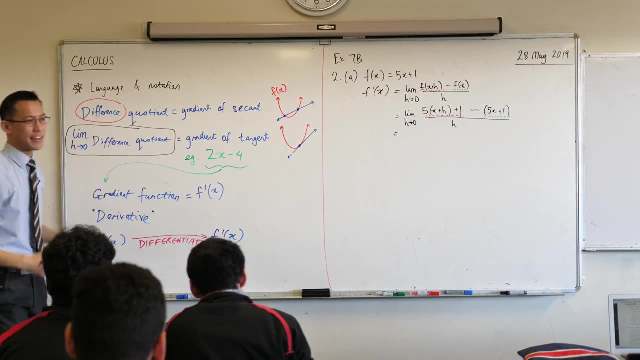 much more complicated. There were squares and all that. This is easy to deal with, right? First thing to write down is: First thing to write down is The limit. Why am I dealing with the limit? Why do I keep writing that down? Look at these two lines. If I don't, 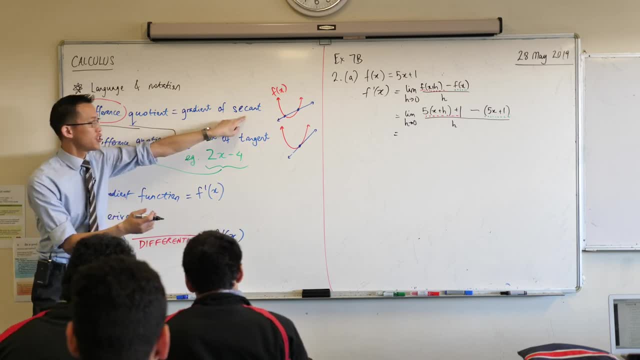 write the limit. what am I working out? I'm working out the difference question, which is a secant right, But I don't want to do that, want a secant. that's just an approximation, Just like us measuring with our triangles. 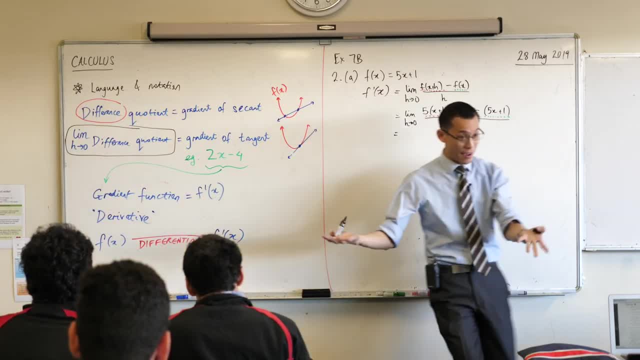 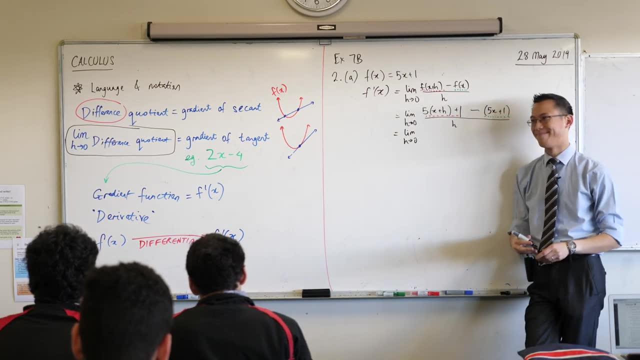 I want something precise, the tangent: Okay, So I have to write: Yeah, Great question. Read the question. So I'm pretty sure it says It'll tell you. It'll tell you what it wants, Though I will point out the only. 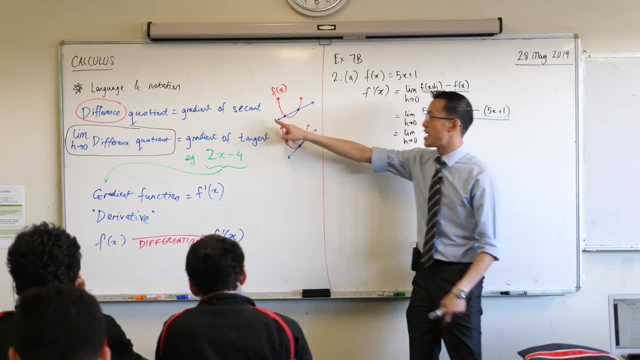 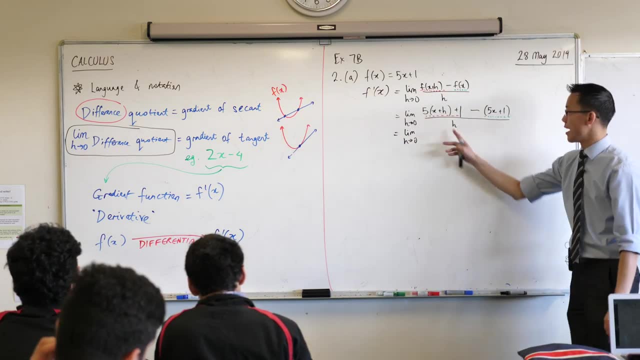 reason we really were talking about secants this morning is because they are the way to get to tangents. Okay, Right, Right, Exactly Okay, Alright, Can you help me out? Can we do a bit of expansion and collecting like terms? 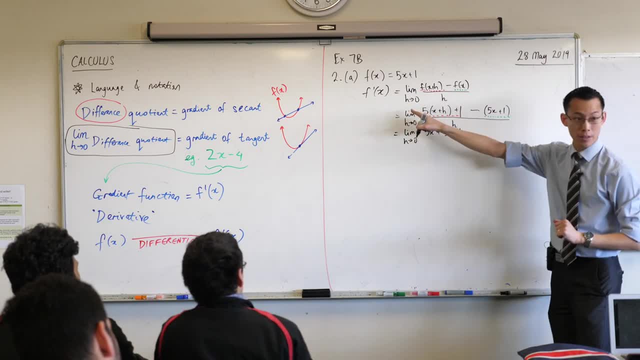 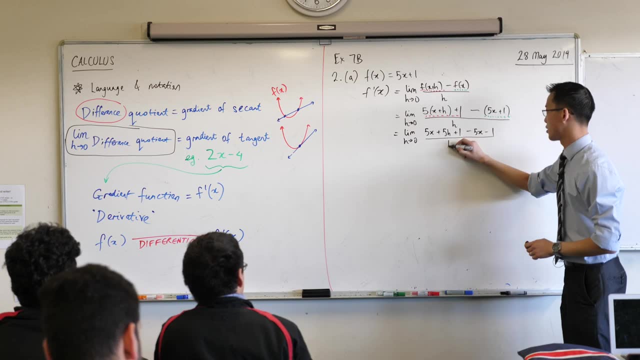 Very good: 5x plus 5h plus 1.. Done with that. Help me out with the second one: Rassand. Fantastic. Now, if we did this right, I should do the whole fraction first. If we did this right, some stuff should cancel right. 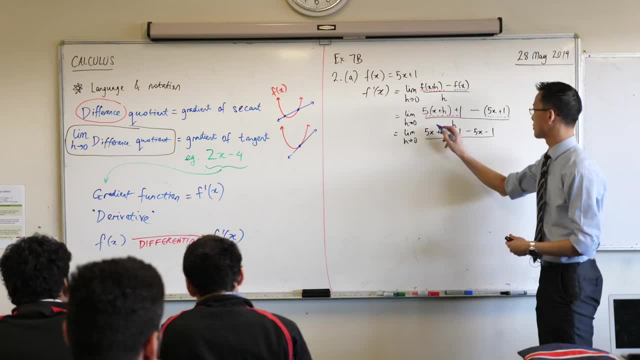 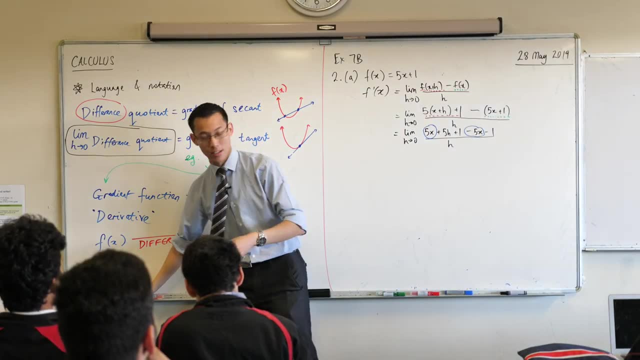 What can you see These guys? By the way, is it obvious enough that I'm trying to help you see this with colours? right, There's lots of stuff that will be more obvious to you if you can just highlight it in this way. 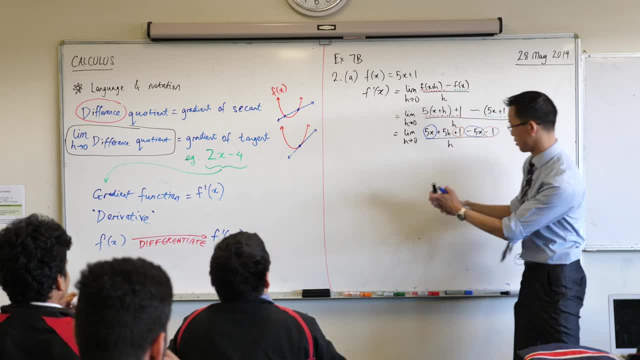 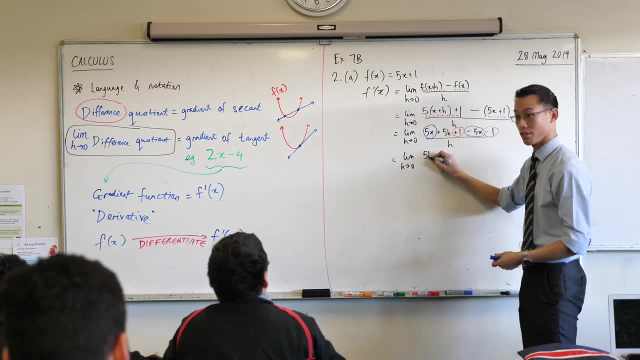 Good, Fantastic. So if you did it right, lots of stuff should cancel and we get left with what? Just the 5h, 5h Over h. So you're like, oh cool, this is the thing I saw before. right, I can get. 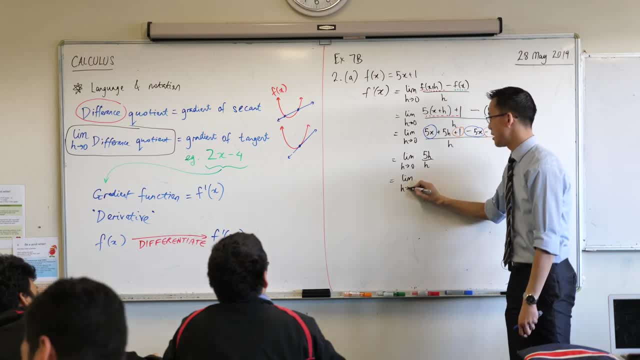 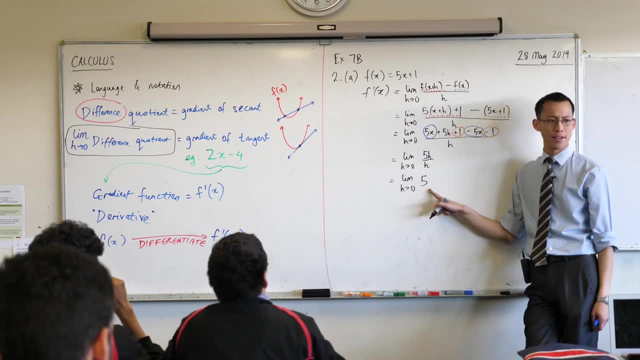 rid of the h's. So I say this Now. at this point you're like: oh, what happens when h gets closer and closer to 0?? What happens to 5 as h gets smaller and smaller? And the answer is: nothing happens to. 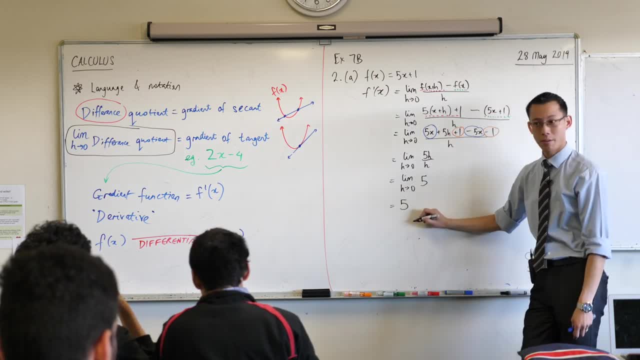 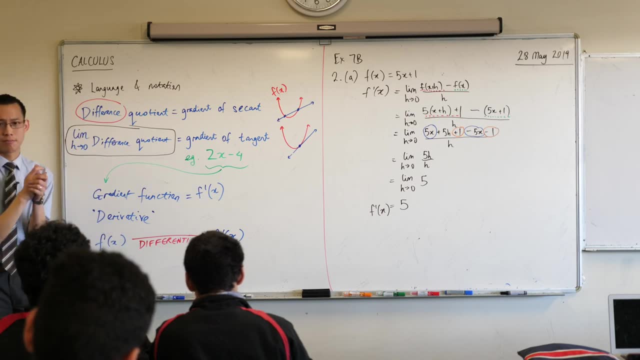 5.. 5 just stays 5.. Now let's just pause, now that we've got an answer, and think about what this means. What is it that we set out to try and calculate? We're differentiating. What does that tell us? What is this thing? 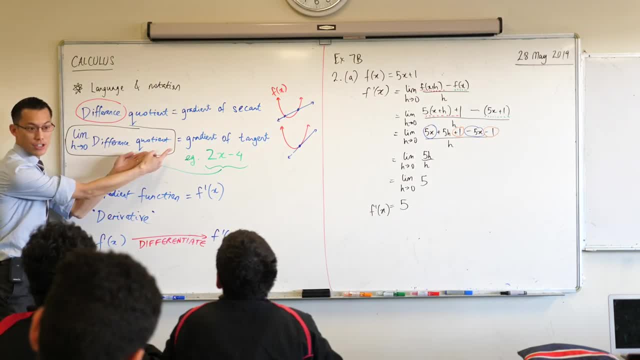 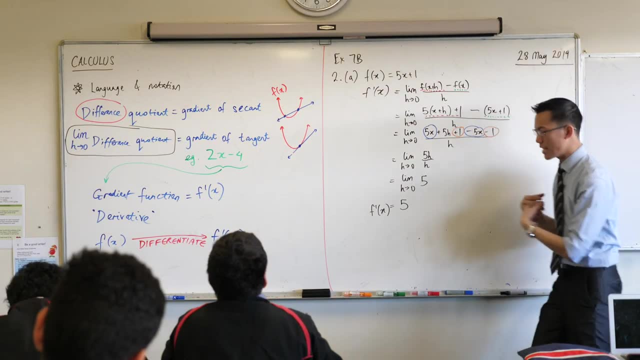 Now it's to do with the tangent. What does it tell us about the tangent, The gradient of the tangent? Now, what this is saying is: you notice, there's no x there, There's no x. So, in other words, whatever value, 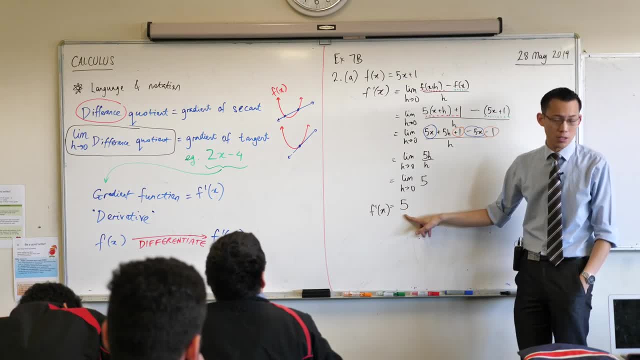 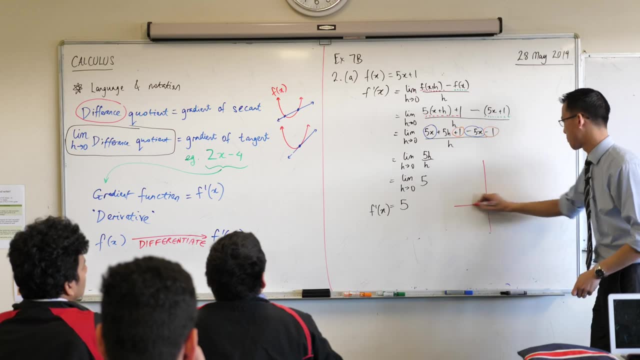 of x. I try out. the gradient of the tangent, apparently, is always 5.. Why is that? What is this object that we're dealing with? This object is a linear graph. It's just a straight line, right? So you're like: 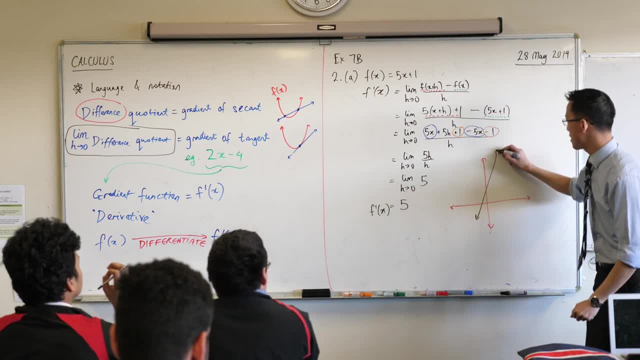 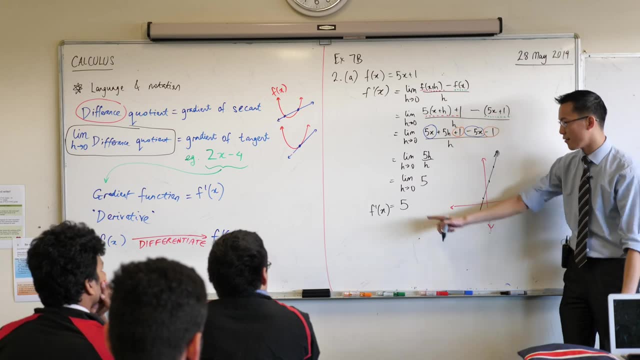 wait a second: 5x plus 1, is this guy right? If you drew in your tangents at every point, pick a point. any point you like, your tangent will always have this same gradient. Make sense? Okay, Now this process. 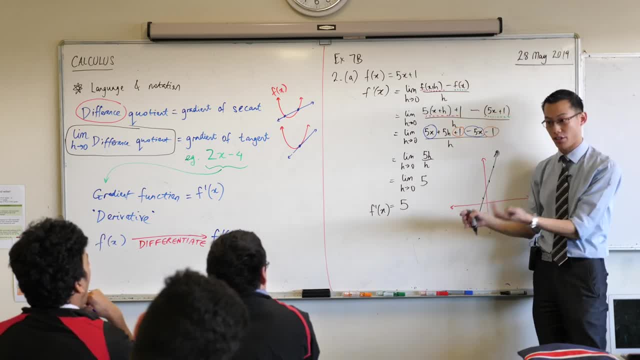 it does look very long. We're going to be replacing this process eventually because it's so long, but you need to know the thing you're replacing it with is doing this in the background, okay. 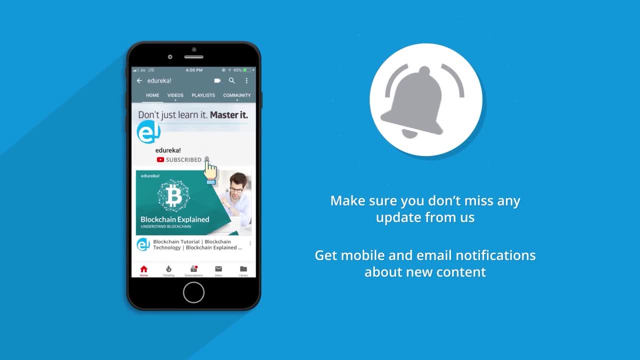 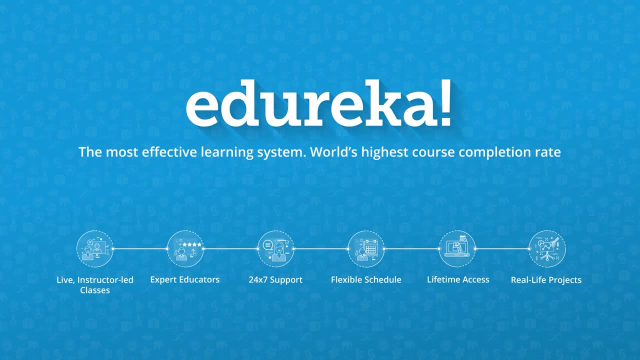 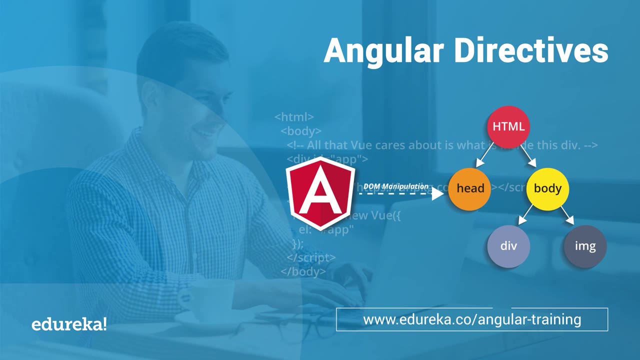 Hey everyone, welcome back to a whole new session from Edureka. My name is Bajeeha, and in this session you'll be learning all that you need to know about Angular directives. So let's take a quick look at what's in store for you all. We shall first begin by